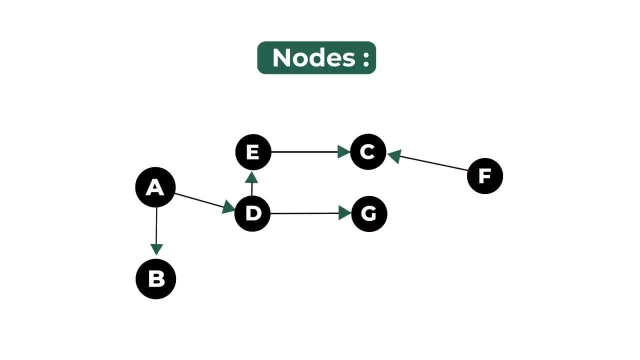 This is how we can think of implementing some of the very popular algorithms of finding shortest paths. Let's talk about how we can travel in between these nodes. Assume you are standing at A, Then A has two options: It can either go to B or it can go to D. right, 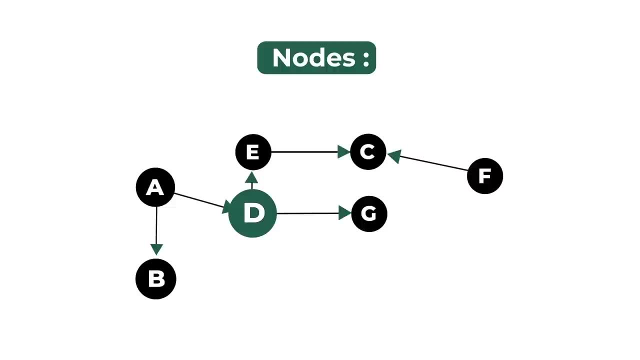 Let's take a step towards D. Once we are here at D, we still have two options. We can either go to E or we can go to D. Let's go to E Now. when we are standing at E, you can notice one thing. 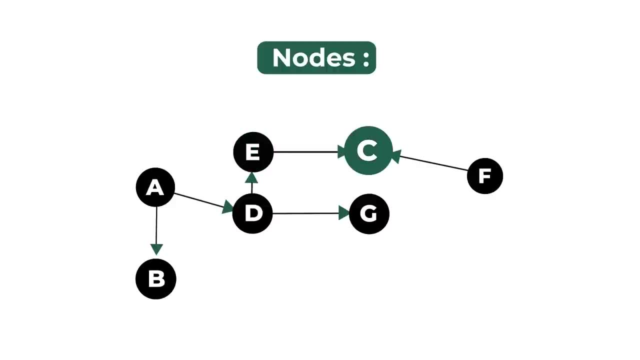 E only has one path to go. That's your C, right. But what if we want to go back to D? Is it possible? No, Particularly. in this graph we don't have any option to go back to the node we are coming from. 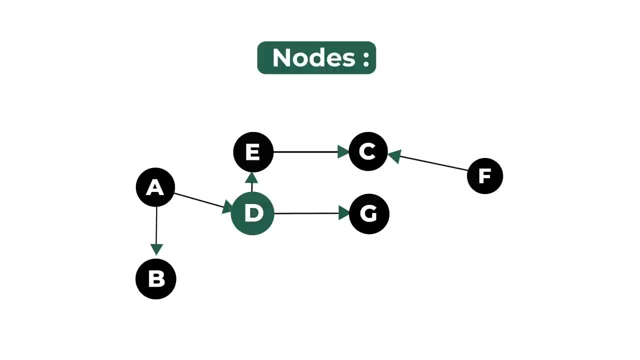 Because this is a directional graph, alright. On the contrary, if we see this graph, this is an undirectional graph. What is the difference? This does not have arrowheads. That means we can even travel back directly to the node which we have travelled from. 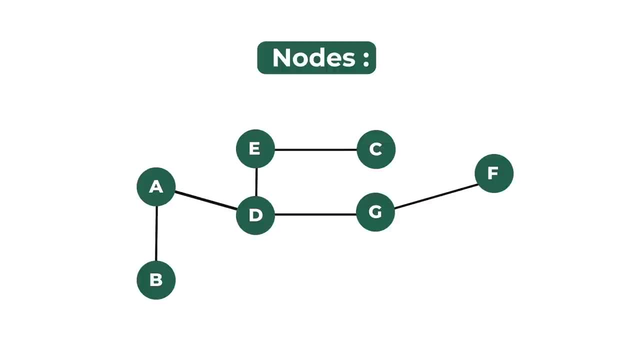 So, assuming in this undirectional graph, if we are standing at E, we'd be able to travel back to D as well, And again then back to A. This is merely a visual representation of a graph. Graph in coding language is going to be a little different. 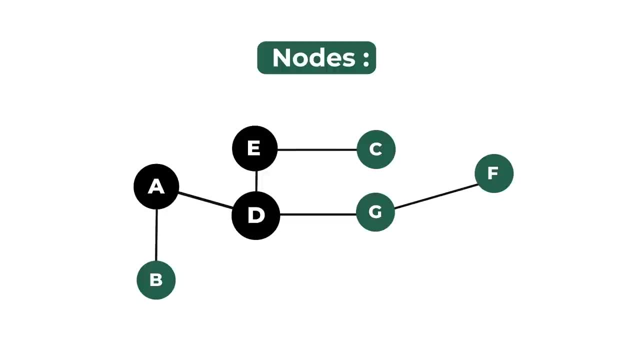 If we have to represent that in any of the programming language, we'd be using a data structure, And most often we use a data structure called as a hash map. We'll be using Python as a language for this video. In Python, we implement hash maps using dictionaries. 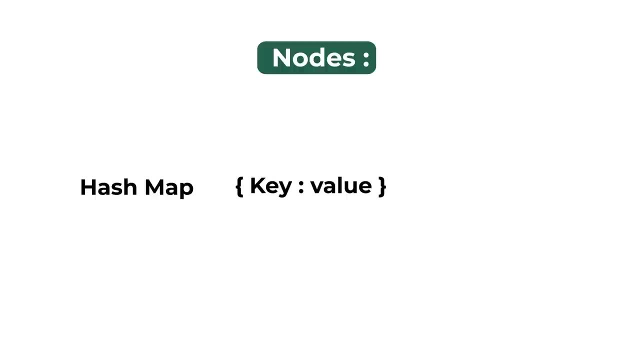 And these are basically key-value pairs And if we talk about drafts, what we are going to do is we will have a dictionary which have keys as the nodes And the value corresponding to every of the key is going to be all the connection it has. 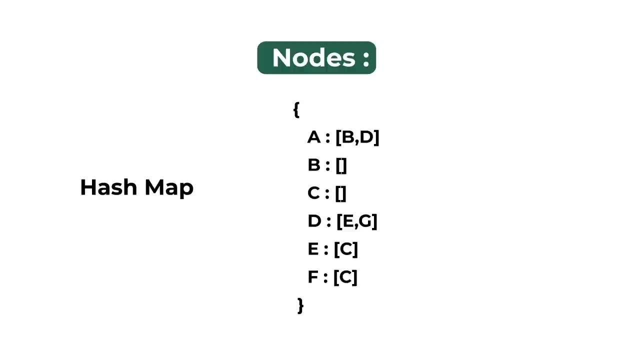 with other nodes. So this format that you can see is actually called as an agency list. Now, as you know how a graph looks like in programming language, we should also know some of the very basic algorithms that we can use in these graphs. 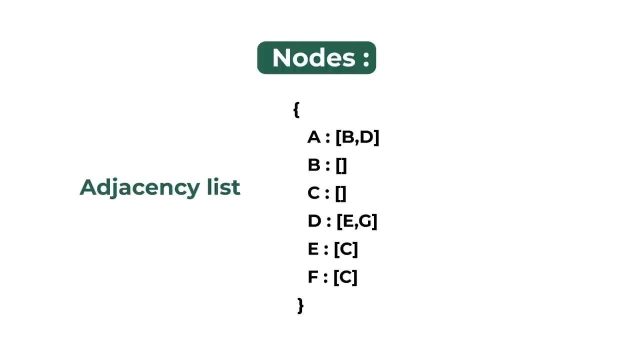 For me and in general, the very basic algorithms that one must know when beginning with graphs. there are two traversal algorithms for graphs. The first one is DFS and the other one is BFS. Let's talk about DFS first. Well, DFS stands for depth, first search. 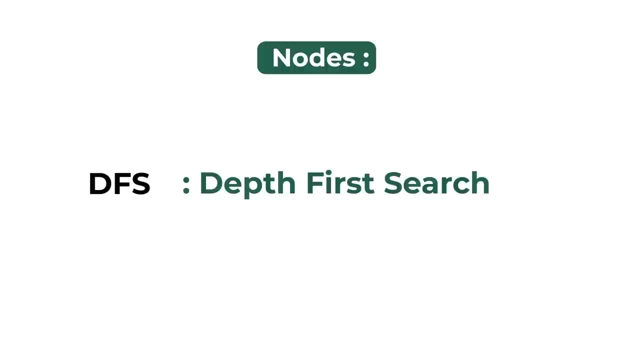 Let's perform DFS directly onto a graph. You can start traversing the graph from any of the node. DFS will be called as a source node. Let's take A as a source node. Now, when we are talking about depth, first search. what we mean is 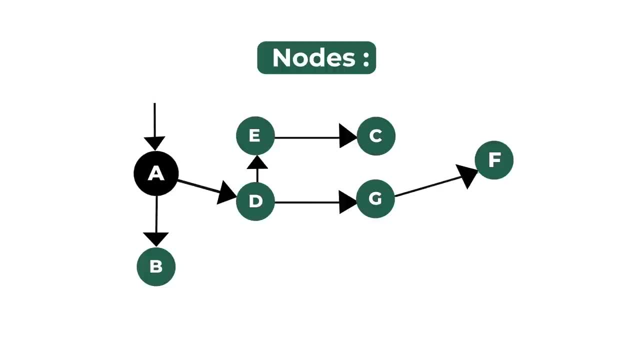 we go in one single direction and we don't get diverted until we have no other option. So when we are at A, we have one choice to make between B and D. Let's go to D. When we are standing at D, we again have two choices. 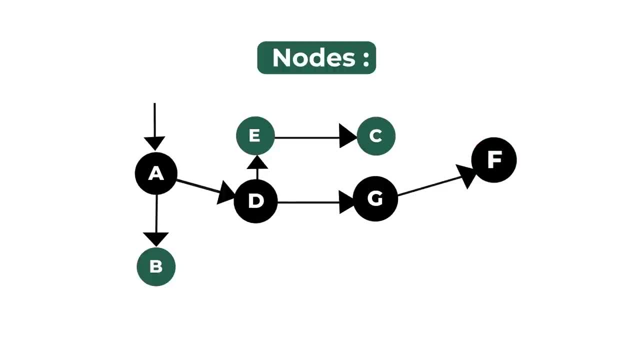 Let's go to G this time. So once we are at G, we only have one choice. So we will track back to G. All the other nodes of G are exhausted. We will go to D now. Well, D still has one path. 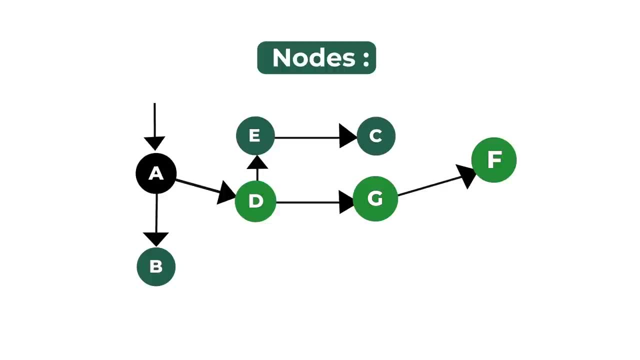 that was not travelled, So we will take up that path. We will move to E And after E we will move to C. Again, we are left with no other option. We will track back to E. We will see that E does not have any other path to go. 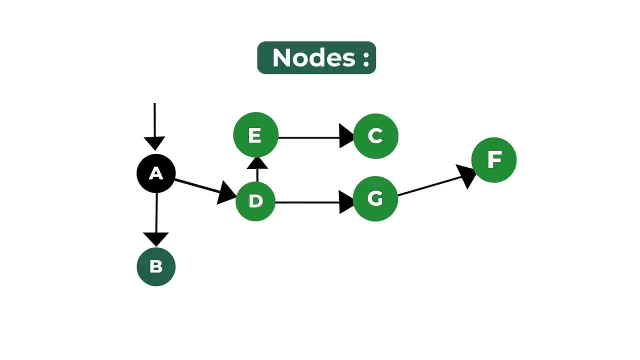 We will again track back to D. This time all the paths of D are also exhausted. We will track back to A. We still have one path to go. That is B. Now we will go to B. This is how we perform a DFS traversal. 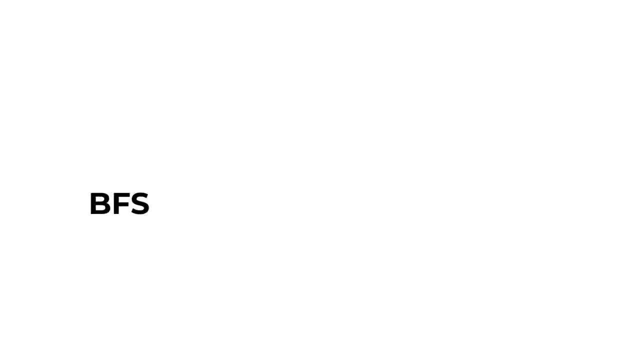 Now let's quickly take a look at BFS. Now let's quickly take a look at BFS. traversal BFS stands for Breadth First Search. Now, in Breadth First Search, what we actually do is when we stand on a node, we travel all of its neighbour. 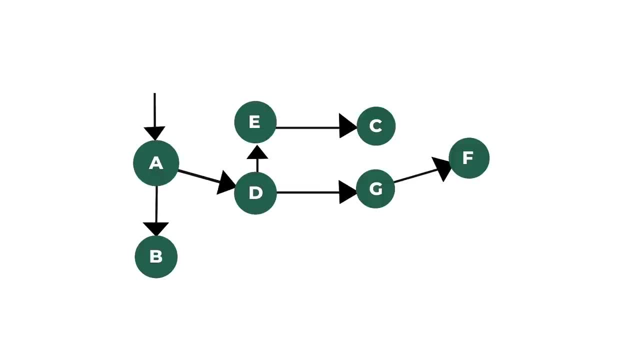 Then we go to each of its neighbour and we travel on to further of the node's neighbour. Let's do that in this graph, Assuming we are standing at A again, the first thing we do is go to one of its neighbour. Let's go to D again. 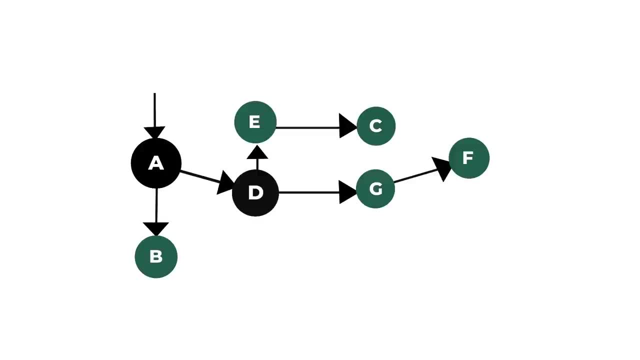 Alright, Once you are at D you have more paths to go to. But because we are travelling in a BFS manner, we will first explore all the other neighbours of A as well. That means the next option is going to be B Now, once all the options of A are exhausted. 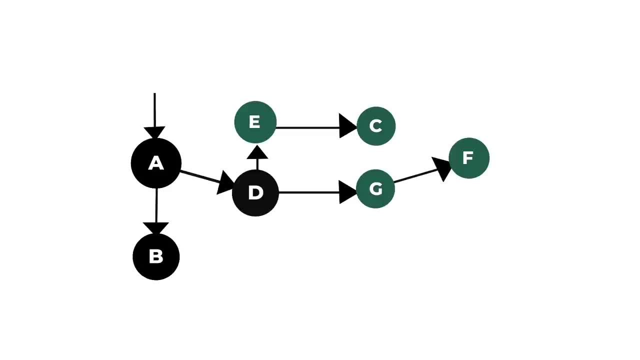 we are going to take up one of its neighbour and then we will travel to that as well. Now we know that D has neighbours. We are going to travel all the neighbours of D. We have E and we have G. Now all the neighbours of G are exhausted. 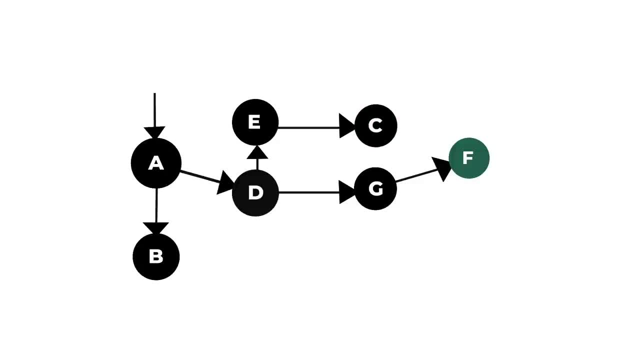 We will take up one of its neighbour. We will take E. We will travel C then. Then we will see: does E have any other neighbour? No, All of the neighbours of E are exhausted. Then we will go to G. We will see all of its neighbour. 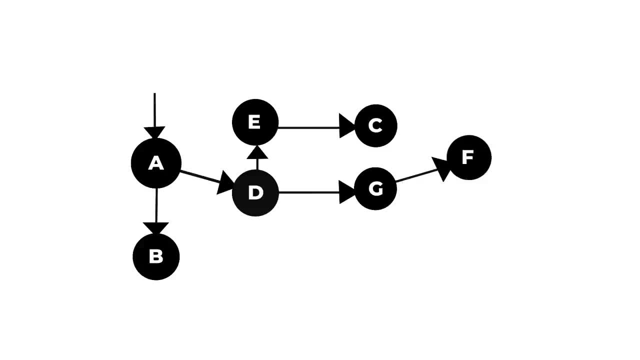 We will go to F And then we will see: all the neighbours of G are exhausted, Yes. All the neighbours of D are exhausted, Yes, And all the neighbours of A are also exhausted. That means we have completed our BFS traversal like this: 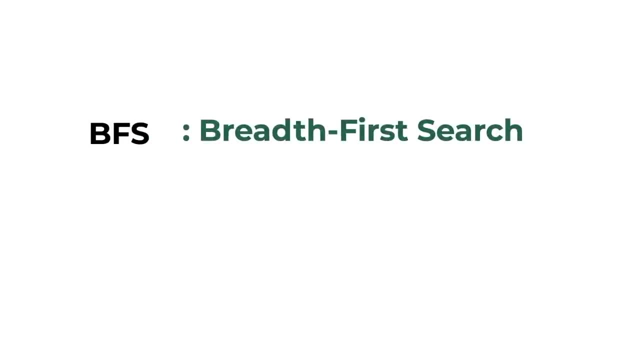 One point that you must know is there could be various possible ways of travelling. a graph: When you are performing a DFS, it might result in different traversals. Similarly, with BFS, if you are travelling in BFS manner, there could be various possible ways. 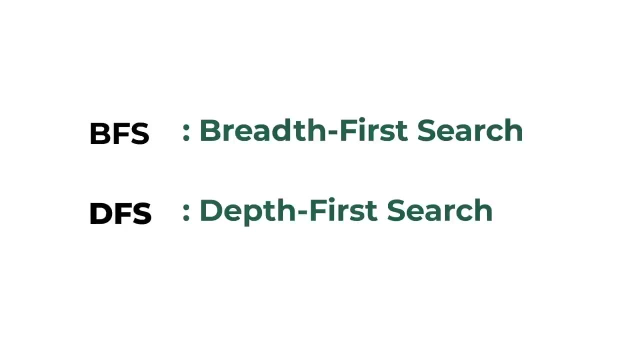 for traversing a graph That depends on each and every choice you make during the traversal. Now that we know both of the traversals, what is actually the difference between them? Well, if we talk about the implementation details, DFS uses a data structure called as. 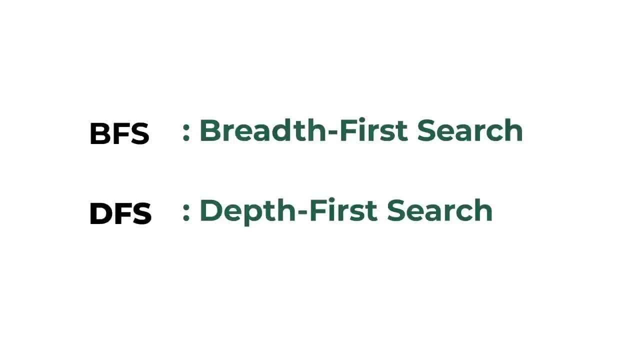 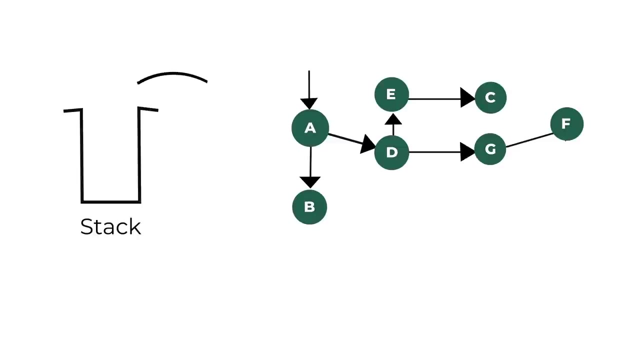 stack and, on the other hand, BFS uses a data structure called as queue. Let's quickly see the implementation of both using the respective data structures. First, DFS: DFS uses a stack. You can assume a stack as a vertical data structure where you can access. 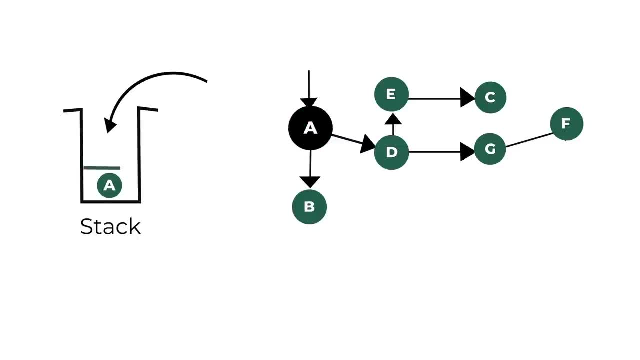 only the element at the top. Like this: Initially, we put on the source node inside the stack. Again, considering A as the source node, the stack looks like this: There is going to be only two operations: Popping the element at the top and then adding all. 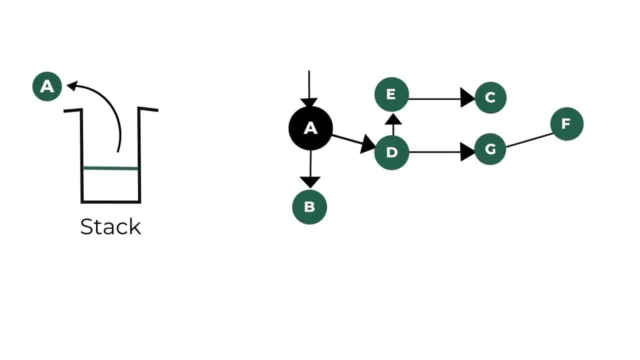 of its neighbours inside the stack. So when we perform it here, we pop A. that means now A is traversed, and the next thing we do is we put on all the neighbours of A inside the stack. This time we put B and then 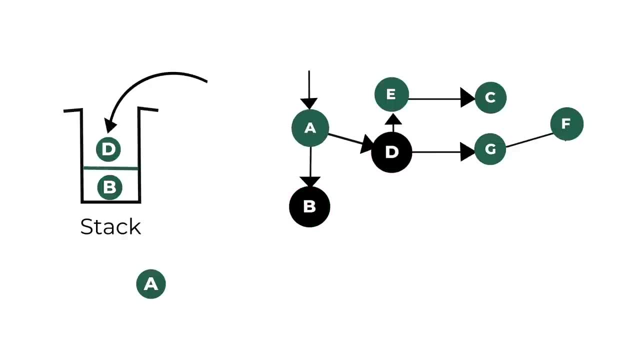 D inside the stack. First step is done. Now in the second, at the top, we have D. We will pop out D After popping that means D is traversed. We have to put on all the neighbours of D inside the stack We can put. 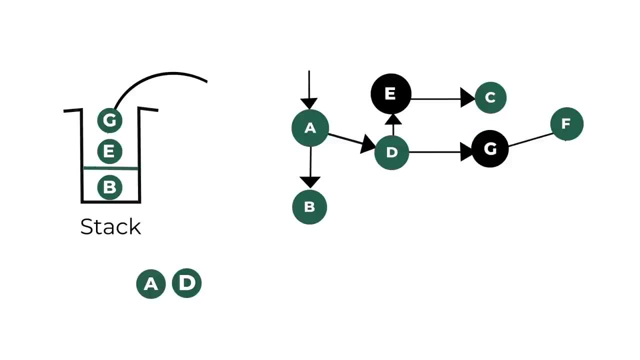 E and G inside it. Now at the top we have G. We will pop G. That means G is traversed, And then we will put on the neighbour of G. That means we have F. now Again at the top, we have F. We will. 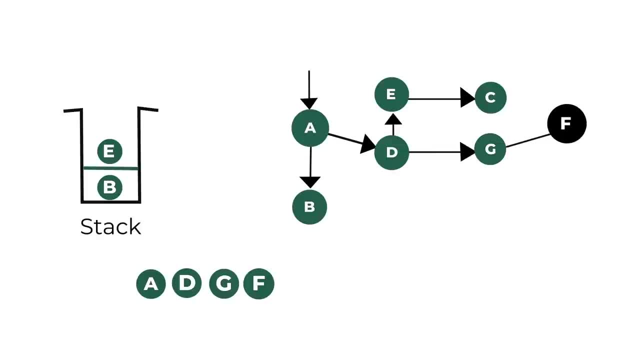 pop F, That means F is traversed. F does not have any neighbour. That means at the top we have E. now We pop E. That means E is traversed. And we put in the neighbours of E, That means we put. 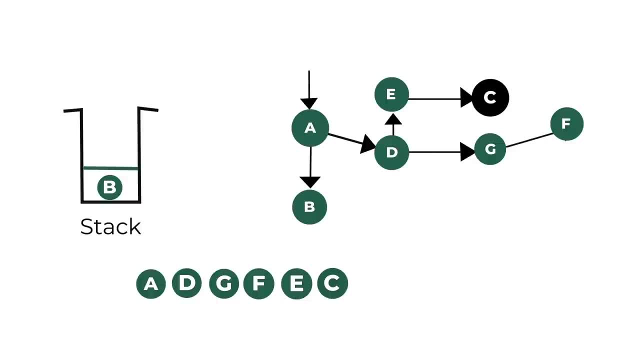 C. now, Once C is popped, that means C is traversed. C does not have any neighbour to put in the stack. As we can see at the top, we have B now We pop out B and we traverse B as well. 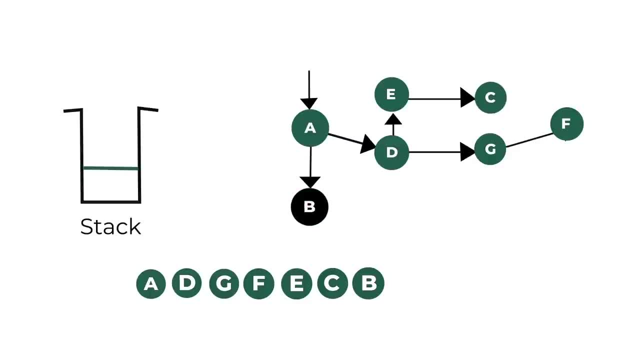 B does not have any neighbours and the stack is now empty. That means the traversal is done. Now coming to BFS. In BFS we use Q. You can think of Q as a horizontal data structure in which we can insert the elements from the rear end. 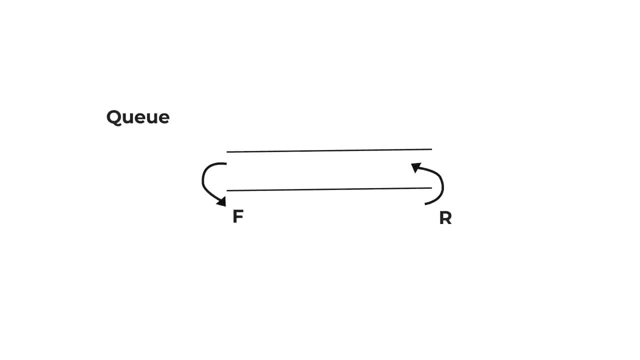 and we delete the elements from the front end Initially again in Q, we put in source: The operations are going to remain same, just the data structure is different. That means we are going to pop the element from the front side and then. 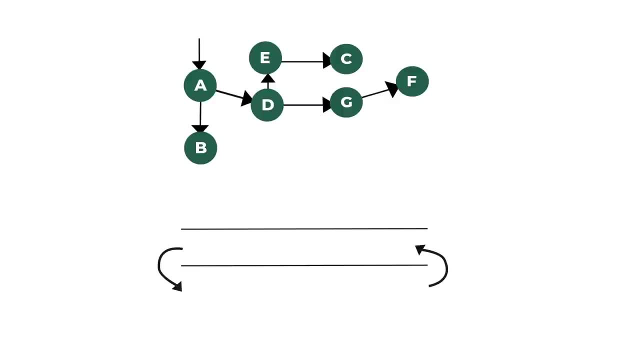 we will put in the neighbours of it from the rear end. So we have A inside a Q. We will pop A. That means A is traversed. We will put inside the neighbours of A. That means B and D. Now this time we have B. 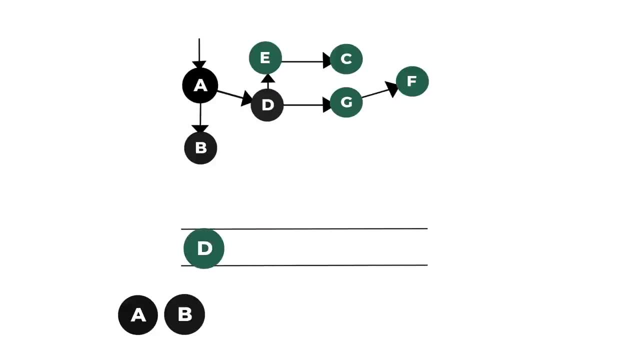 We pop out B, B is traversed. now We put in the neighbours of B, We do not have any neighbours of B. That means we are going to proceed. Now we have D, We pop out D. That means D is traversed. 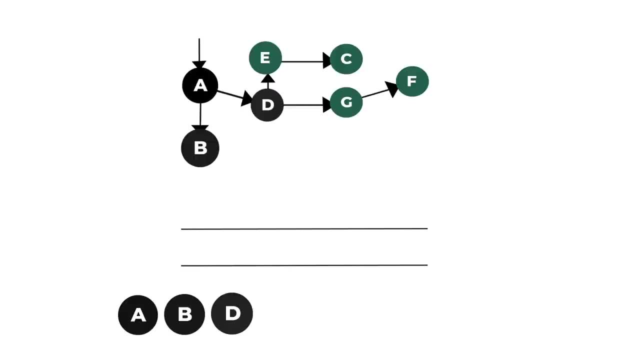 We put in the neighbours of D. That means E and G. Now we have E at the front end. We are going to delete E. That means we are going to pop E and E is traversed. We put in the neighbours of E. 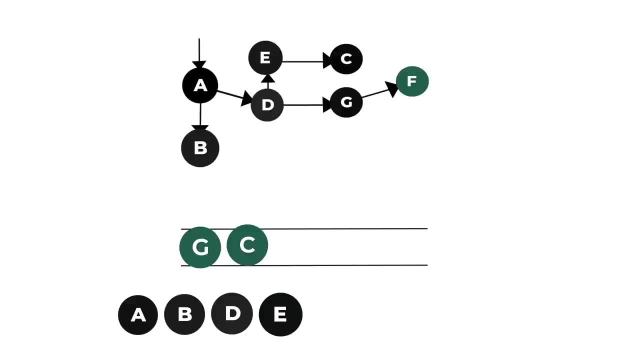 That means we put in C. Now we have G, We pop G and G is traversed. And we put in the neighbours of G. That means F. Now we have C, We pop C and now we have traversed C as well. 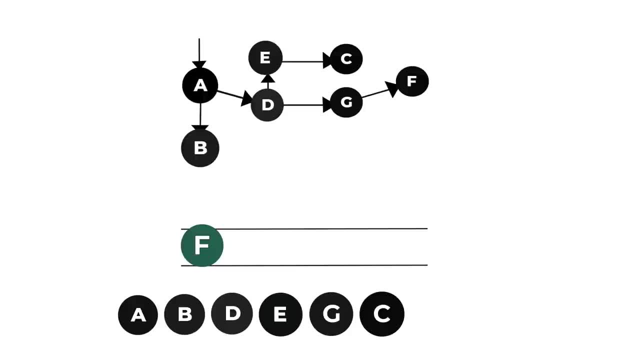 The last left inside the Q is F. We pop F, F is traversed, F does not have any further neighbours And the Q becomes empty. That means this is the end point of the algorithm and the BFS is done. Now let's quickly see. 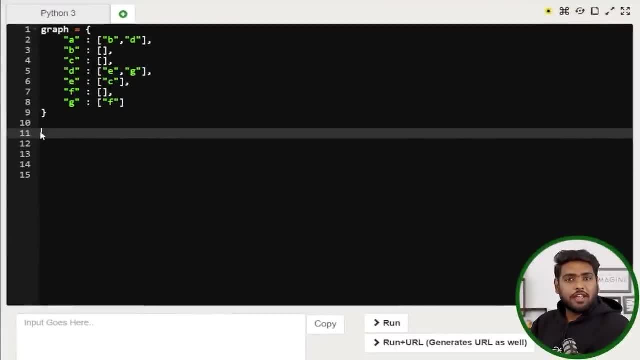 the coding implementation of these two algorithms. Here we have created the same graph that we have seen. Now let's code a DFS function for it. So what are the two things we need for a DFS to work? The first thing is the graph itself. 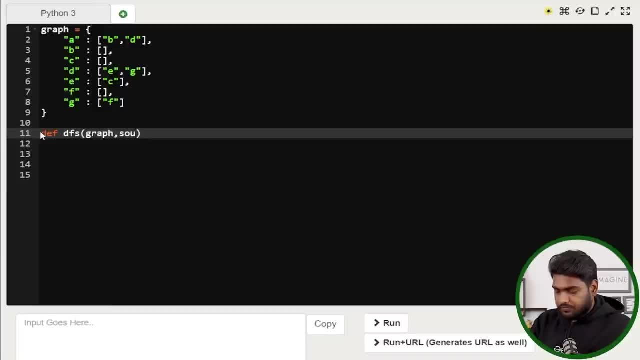 and then we need source. The second thing is the DFS to work. We use a stack in a DFS function, So I'm going to initialize a stack In Python. I'm using a list and I'd be using only one end of the list. 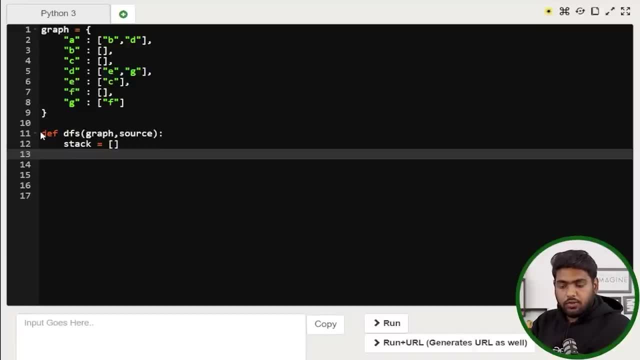 so it would act as a stack. Initially, we put the source node inside the stack, So I'm going to do that like this. Once this is done, now we have to repeat the two steps. right, What are those steps? I'm going to pop the value that is present inside the stack. 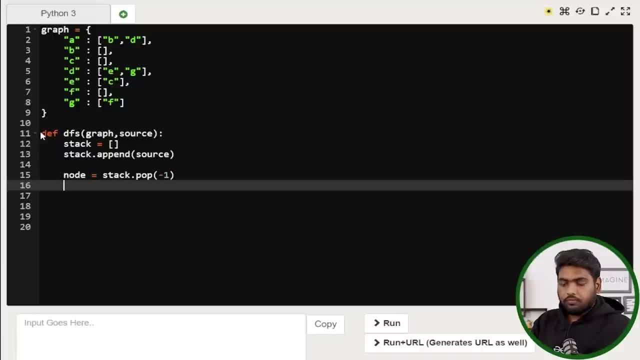 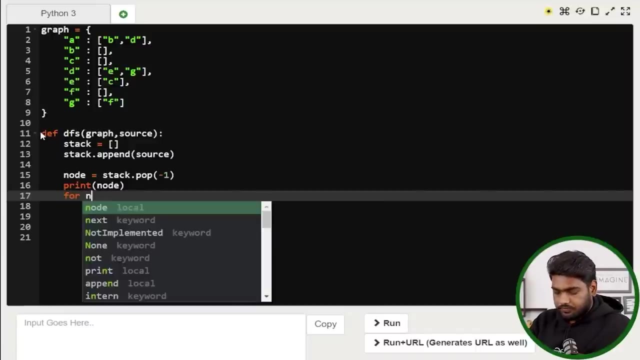 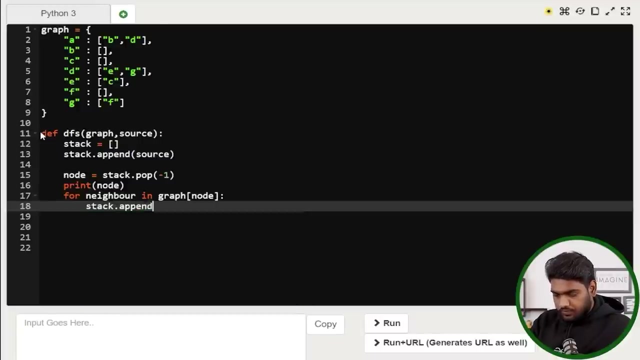 Alright, Then I visit it. So for visiting, I can simply print it Right. And the last step is to put in all the neighbors of that node inside the stack Right. These are the steps, And till what point we have to do these steps. Well, as we have. 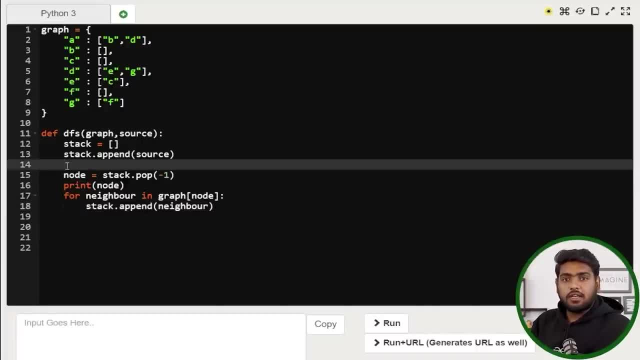 already seen in the illustration. we are going to do all these steps till this stack is empty. This is simply a very basic DFS function. Now, let's call this DFS function. We have to give the source node. So, as we were taking A as a source node, let's take A again. 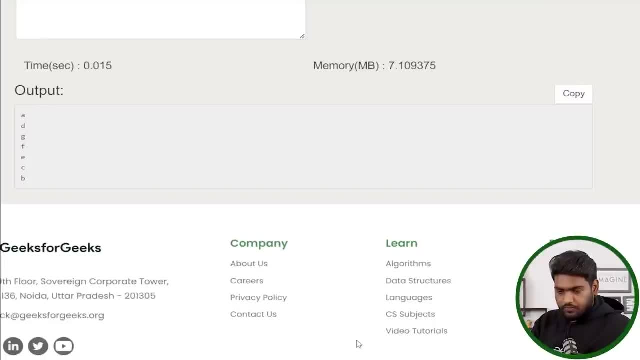 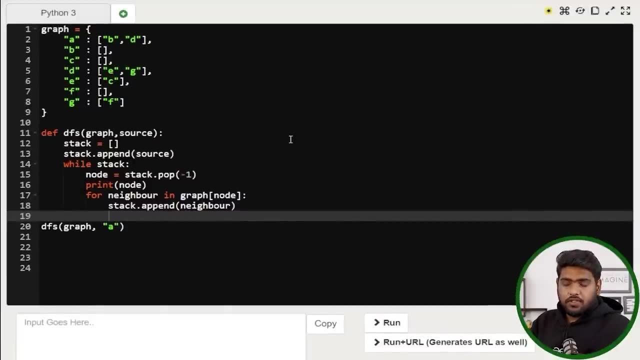 Let's run the code. Okay, Here we have the DFS traversal of our graph. Now let's talk about the BFS traversal. I'm going to make a very few changes in this code and that will then act as a BFS function. The very first thing, let's change the name of it. 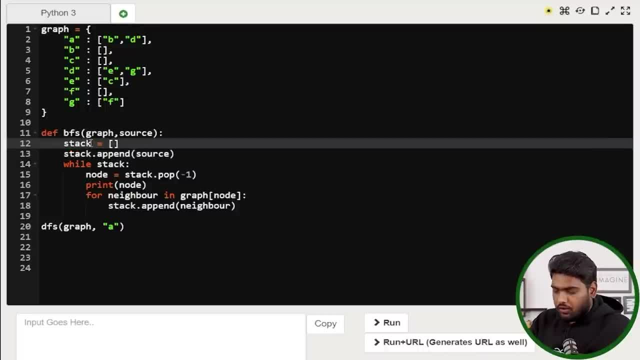 And then, just for the sake of clarity, I'm going to rename the variables. Okay, Now I'm just calling the same list as Q And I'm going to be implementing the aspects of Q to it. So I'm going to be appending it from the rear end, but instead of popping it from the rear, 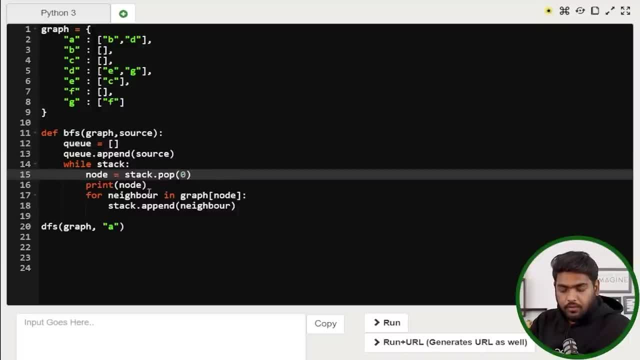 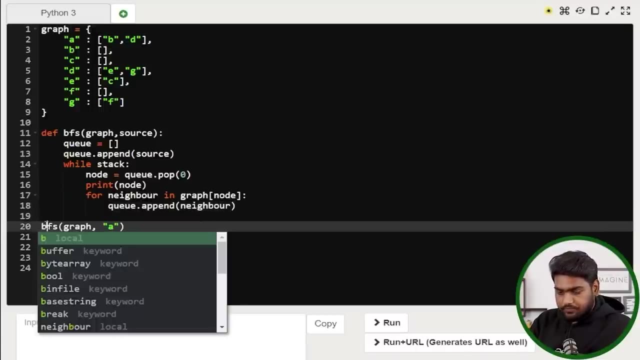 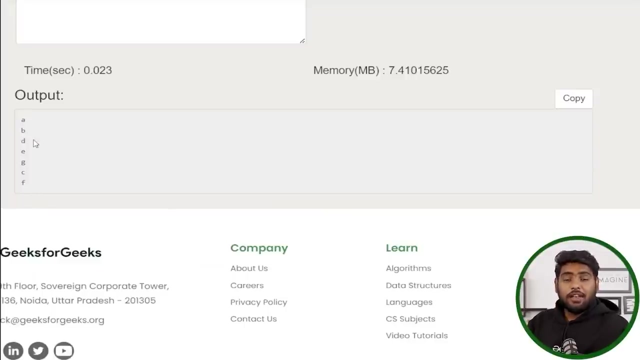 end, I will pop it from the front Right And every other thing is going to be same Right. Now let's call this function as well. So here we have the BFS traversal of the same graph. I believe this video was very helpful for.